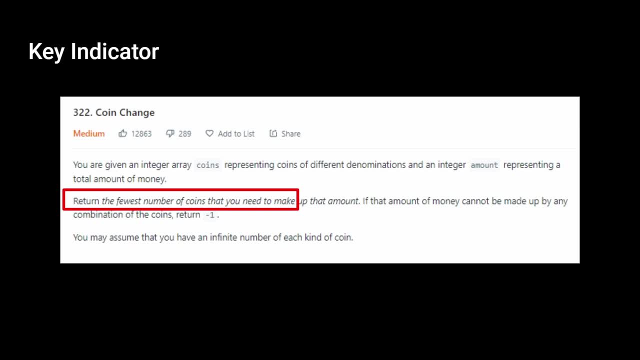 we have to use the fewest number of coins possible. Whenever I see the word few or the words fewest, what that indicates to me is that we need to perform some sort of optimization, And generally, optimization problems can be solved with either a greedy approach. 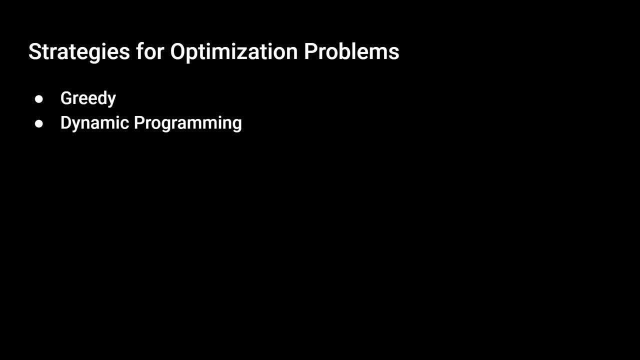 or a dynamic programming approach. Now, in order to determine if a greedy strategy works or doesn't work, one strategy I like to use is to actually generate an example that can disprove that the greedy strategy would work. So one example I generated is with the coins one, five and seven and a target amount of eleven. So 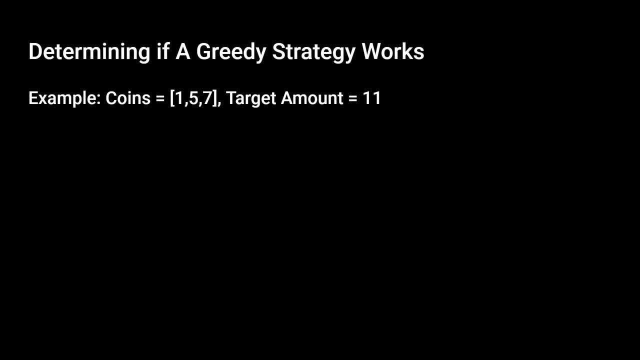 if we were to take the greedy approach. what we do is we start off with the biggest number that is currently less than or equal to the target amount, and what we do is, as we deduct from the target amount, we keep grabbing the next available highest number until the target amount. 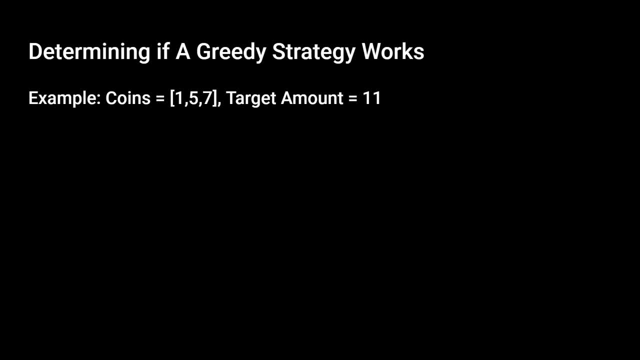 has been reduced to zero, And so if we were to do this, what would happen is we'd start off by grabbing seven and then, after that, we grab seven, the remaining amount would be four. So that means we can no longer grab seven, we can no longer grab five, we can only use ones. So after 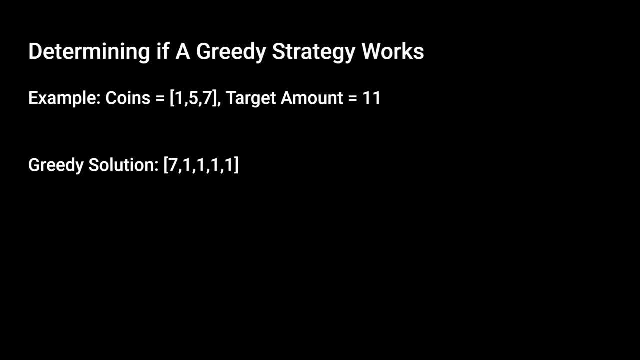 that we would grab four ones so that we can generate a set of coins that sum up to the target amount of eleven. Now the actual solution is to use two coins with the value of five and one coin with the one value of one. So this indicates that the greedy strategy doesn't work. 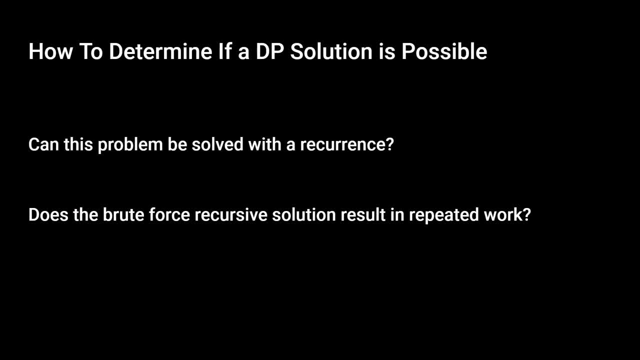 So, in order to determine if a dynamic programming solution is possible, we need to answer two questions: First, can this problem be solved with a recurrence? And second, does the brute force recursive solution result in repeated work? If the answer to both these questions is yes, then we can use dynamic programming. 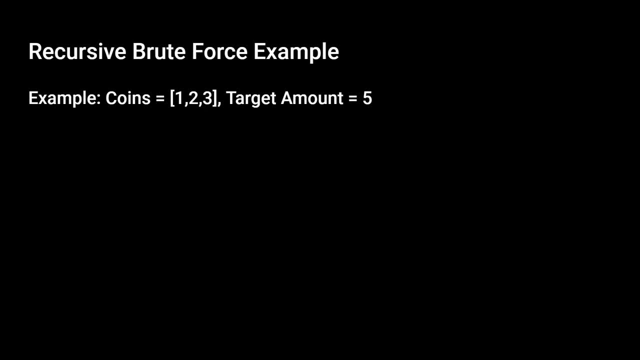 So here's an example of how we would solve the question with a recursive brute force solution. What we do is we use a top-down strategy, which means we start at the target amount of five and we'll work backwards to see how many coins it'll take to get from the target amount of five to our starting amount of zero. 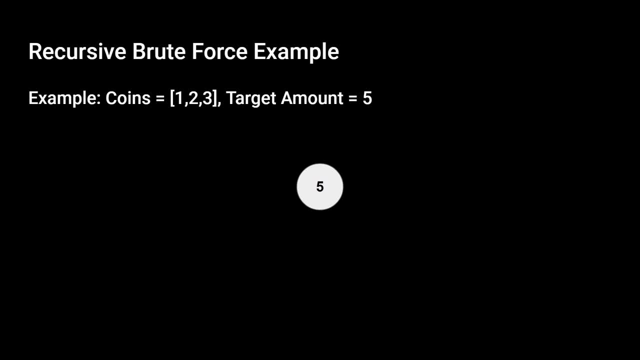 So, starting with five, what we're going to do is we're going to take the coins one, two and three and we're going to deduct them from five, So that will yield the amounts four, three and two, And from then on we will continue. 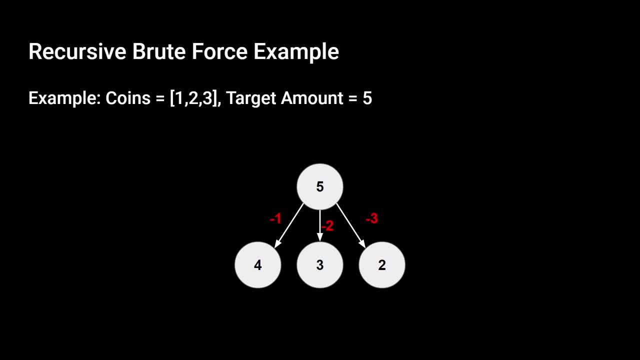 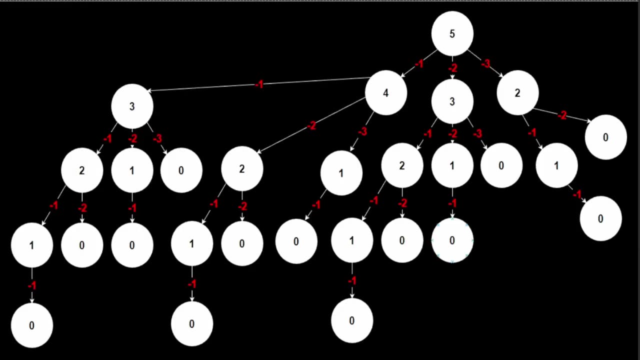 from these remaining amounts until we get to the initial amount of zero, And then we'll just count up how many coins it took, and then the minimum amount of coins it took to get from five to zero will be our answer, In order to make this tutorial more concise. 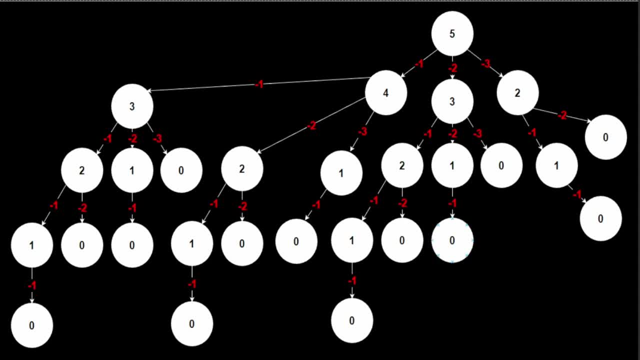 I went ahead and completed the tree. that would result from a recursive brute force solution. This essentially represents all the different ways we can go from the target amount of five to the amount of zero Based on this diagram. the minimum way to sum up to five is to use two coins. 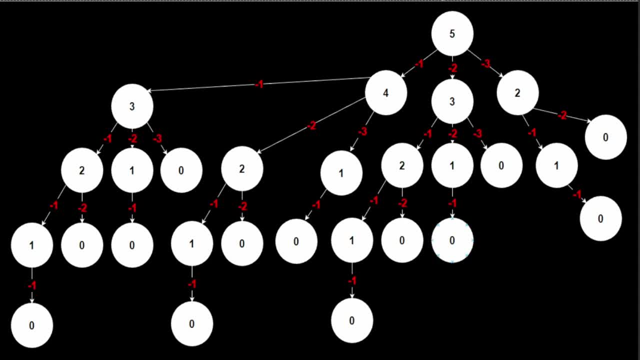 We could just use the coin with the value three and the coin with the value of two, as is shown here. So now that we've determined that we can solve this problem recursively, let's see if there are areas where we're repeating work. 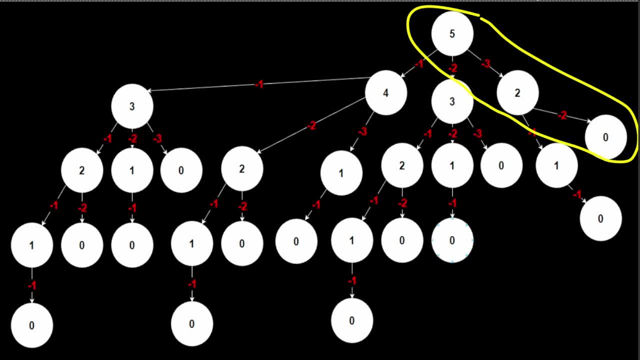 So immediately, two areas that pop out to me is the work we do to see the minimum amount coins needed for the subproblem of 2, because we calculated it once there and then we calculated it here, and we calculated it here and then we calculated it here. 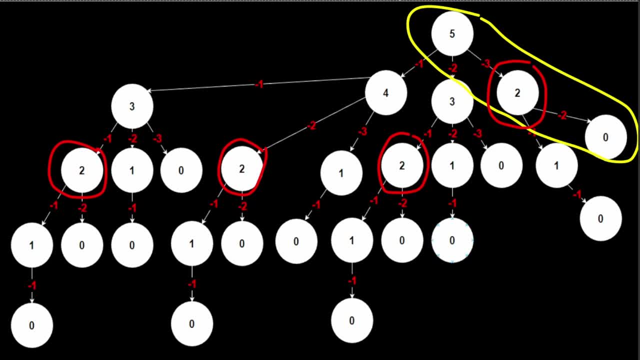 And then, if you look carefully, we're also repeating work for our calculations for 3, because we do it here and then we also do it again here. So, because we are solving the same subproblem over and over again, we can use memoization or dynamic programming to solve this question. 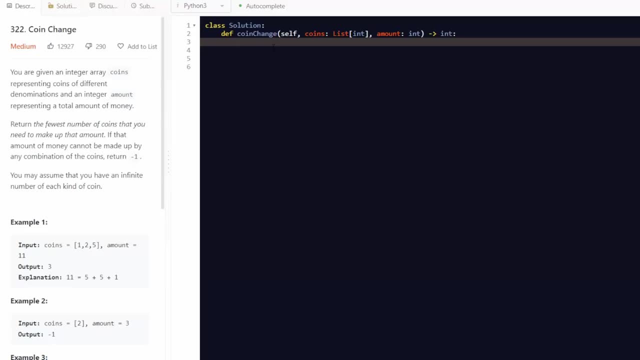 Let me show you the memoization approach first. So, in order to start coding our recursive solution, what we're going to do is we're going to start defining a function that's going to perform all the recursive work, So we're going to define a function called recurrence. 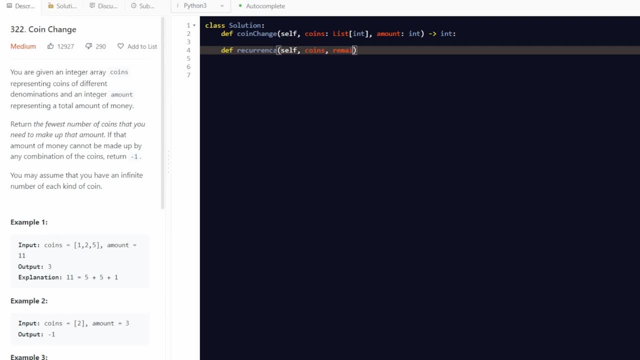 It's going to take in a list of coins that we have access to. It's also going to keep track of the remaining amount. Now, if the remaining amount is equal to 0, then that means we have 0 coins we need to apply to the remaining. 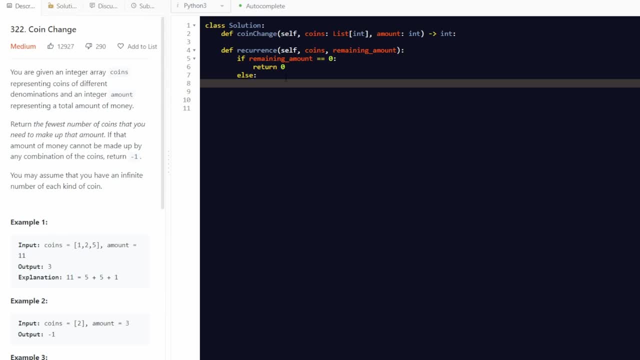 Otherwise, if the remaining amount is non-zero, then we need to keep track of the minimum amount of coins we need to solve for the remaining amount. We're going to use a very high value- infinity- to keep track as a placeholder for the minimum amount of coins needed. 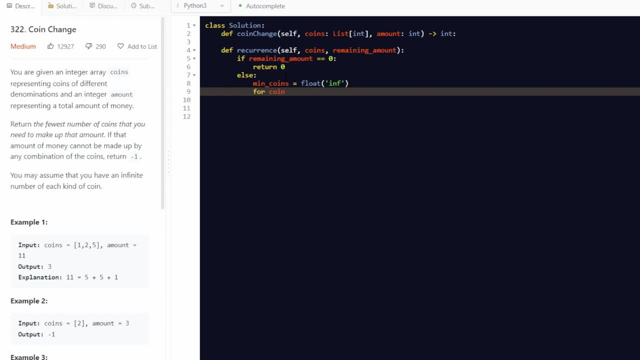 Now what we're going to do is we're going to iterate through all the coins And basically we're going to try to use all the coins to solve for the remaining amounts. Now, if the coin is less than or equal to the remaining amount, 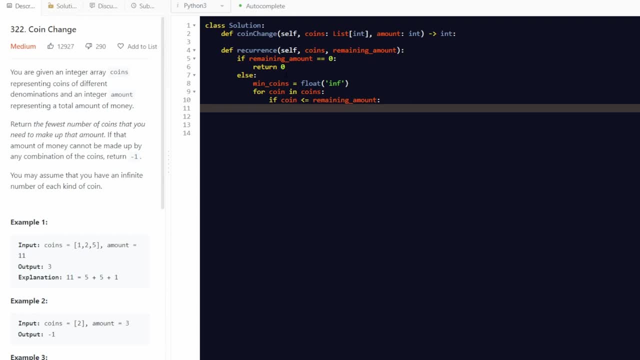 we can use it And how we're going to use it is basically we're going to see if, by taking that coin or the current coin, we're considering if that will result in a solution that uses the minimum amount of coins. And so what we're going to do is we're going to set mincoins to the minimum. 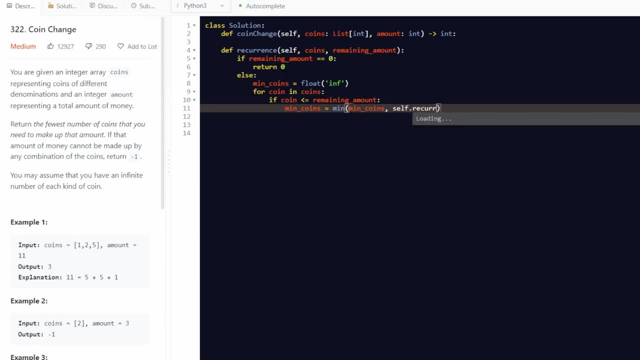 between the current solution and the solution we get by making the next recursive call. And so, in order to make the next recursive call, And so, in order to make the next recursive call, we're going to call the function, We're going to deduct the remaining amount by the coin we're using. 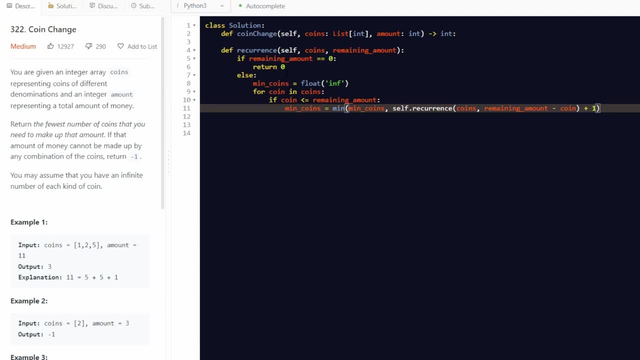 And then we're going to increment, whatever the answer is, by one to indicate that we've taken that coin that we're currently considering. Once this loop terminates, we've considered all the coins And then we're just going to return the value that's being tracked in mincoins. 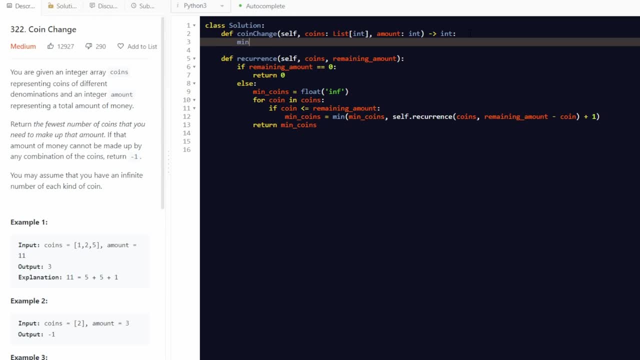 Then we can call the recursive function in our main function in order to get the answer. So mincoins is going to be equal to the recurrence We're going to pass in the list of coins We're going to pass in the target amount. 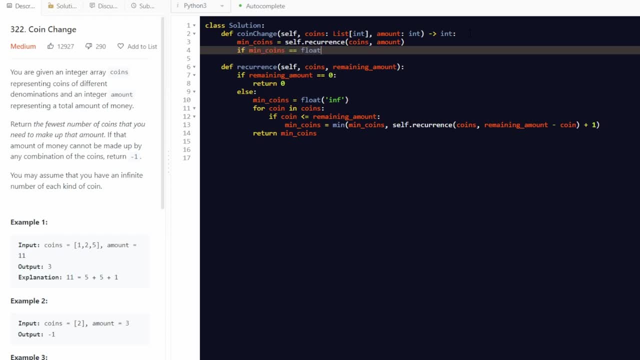 And then what we're going to do is: if mincoins is equal to float infinity, then we need to return negative one, because that indicates that the combination of coins we have aren't able to sum up to the target amount. If it's not infinity, then that is going to be the minimum number. 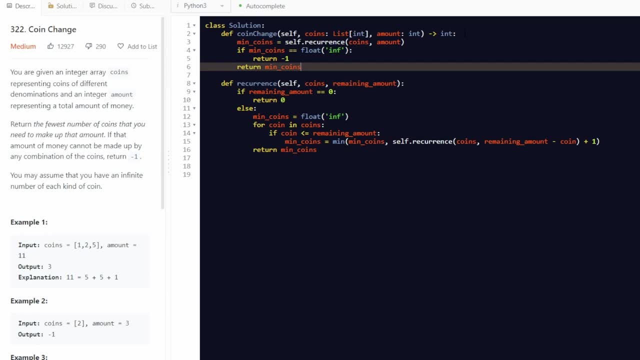 of coins needed to sum up to the target amount. Now, this is just the brute force recursive solution. What we can do to make this more optimized is to store all of the solutions to the different recursive calls we've encountered, And this process is called memoization. 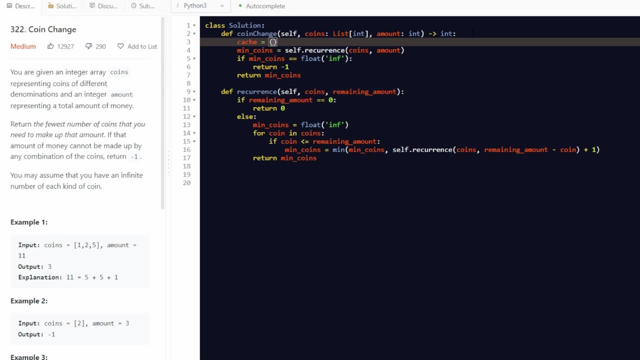 And so what we're going to do is we're going to declare a cache. That's just going to be a Python dictionary, And the key for this is going to be all the remaining amounts we encounter, And the value will just be the mincoins needed. 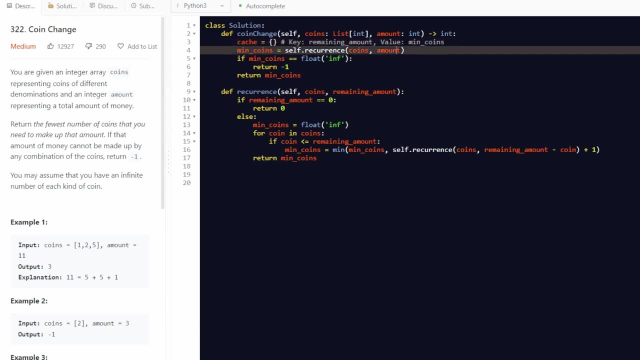 And then what we're going to do is we're going to use the cache to solve for that remaining amount, And so we're going to modify all of our method signatures to take in this cache. And then, in order to use the cache, what we're going to do is, every time, 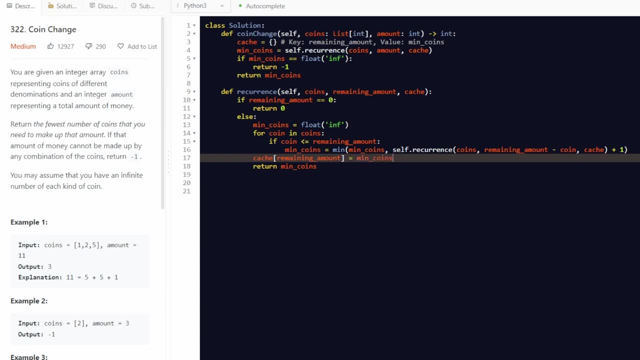 we calculate a solution, we're just going to set remaining amount for the cache to be equal to the mincoins And then, if we ever make a recursive call for a remaining amount, we're going to return the solution to the cache and return the solution from the cache. 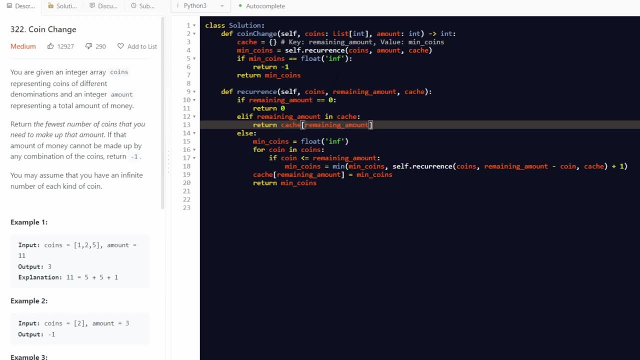 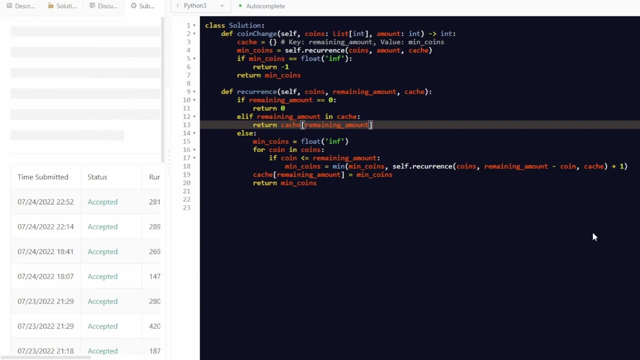 That way, we're not repeating any work and it makes our algorithm a lot faster, And so when we submit this, we'll see that it's able to finish. And then this is the memoized solution, And what I'm going to do next is I'm going to show you how the dynamic programming solution works. 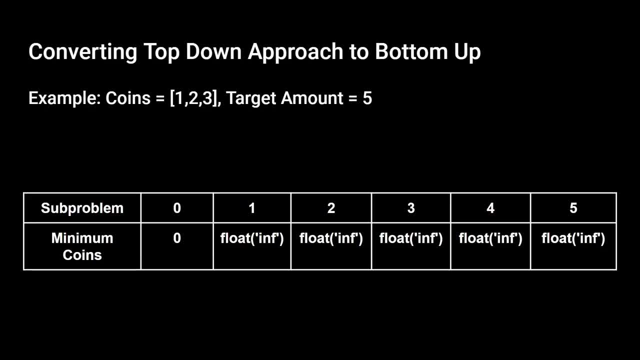 In order to convert the recursive solution to a cache. we're going to use the recursive solution to a dynamic programming solution. We'll reuse a lot of the concepts from the recursive solution. The only difference is the base case from the recursive approach is now the starting point for the DP approach. 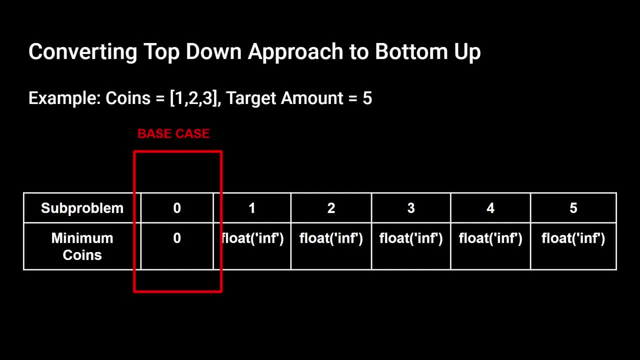 The different subproblems of the DP approach will build upon previously solved subproblems. Let's walk through the DP approach and see what will happen when we apply it to this example, where our coins are 1,, 2, and 3 and the target amount is 5.. 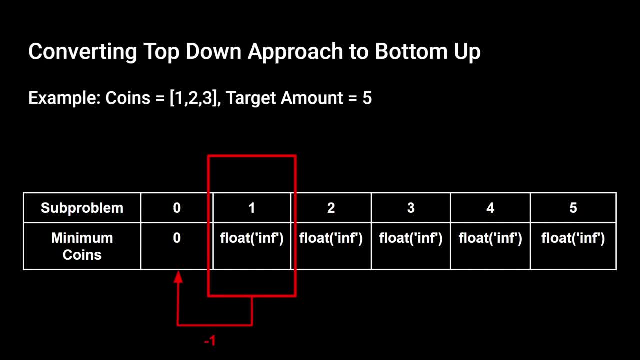 To sum up to 1, the only coin we can consider is the coin with the value of 1.. We cannot use the coins 2 or 3, since they exceed the sum we are solving for Working backwards. the only way to get from subproblem 1 using coin 1 is to have started from the subproblem 0.. 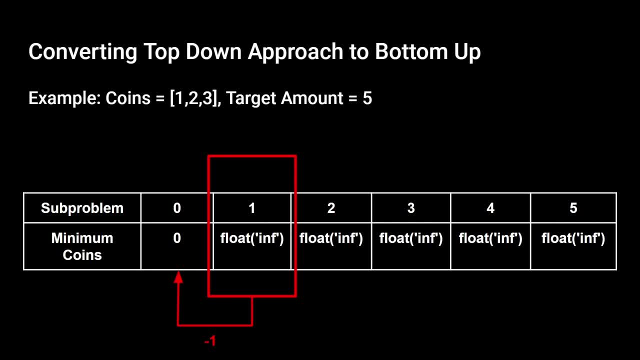 So we'll use the answer from subproblem 0 incremented by 1 to account for the coin we're using. This results in 1 coin being the minimum amount of coins needed to sum up to 1.. In order to solve for the subproblem 2,, the coins we have access to are the coins with the value of 1 and 2.. 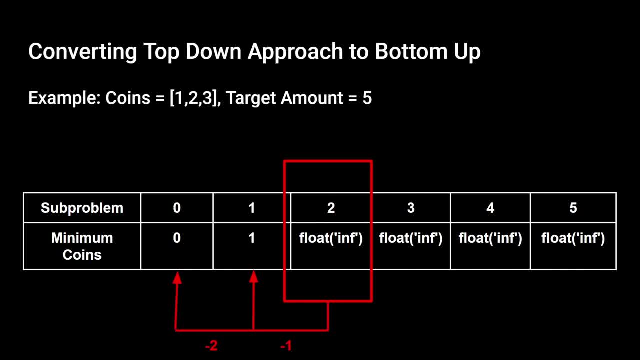 Using the coin with the value 1, we can get to subproblem 2 from subproblem 1.. Using the coin with the value of 2, we can get to subproblem 2 from subproblem 0.. The solution for subproblem 0 has the least amount of coins. 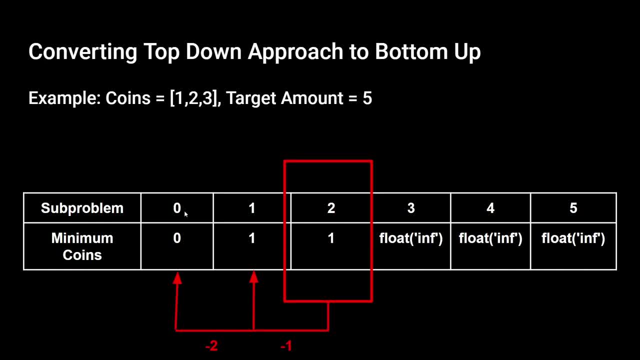 so we'll take it and we'll increment it by 1.. This results in subproblem 2 having the solution of 1.. In order to sum up to 3, we consider all the coins. Using the coin with the value of 1, we can get to subproblem 3 from subproblem 2.. 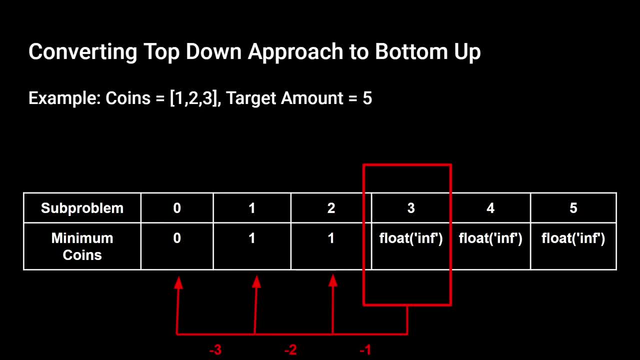 The coin with the value of 2 will allow us to get to subproblem 3 from subproblem 1.. And the coin with the value of 3 can get us to subproblem 3 from subproblem 0.. The solution for subproblem 0 results in the least amount of coins. 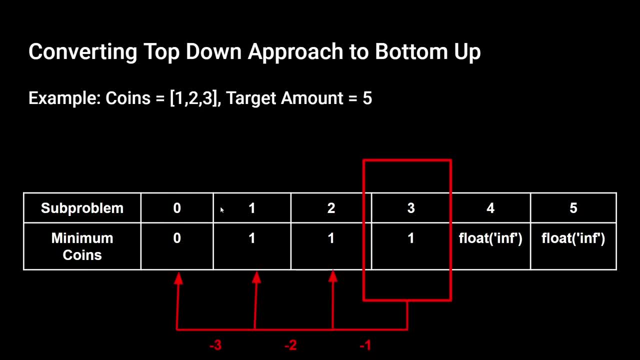 so we'll take its solution and increment it by 1.. This results in 1 coin being the minimum amount of coins needed to sum up to 3.. We will continue this process to solve for 4.. And that will result in subproblem 4 requiring 2 coins. 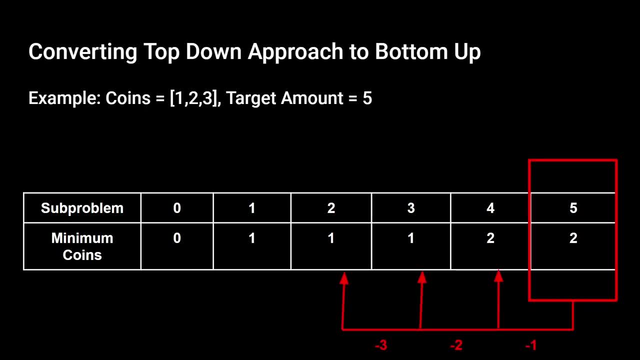 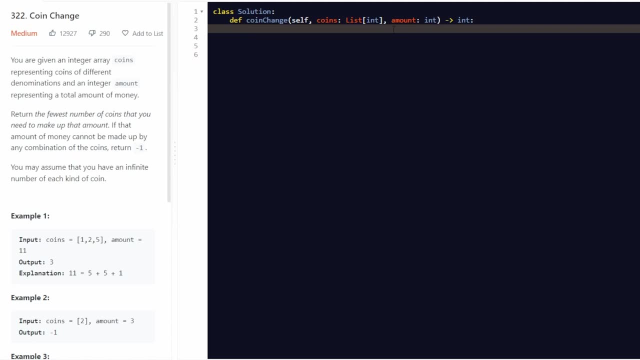 And we do the same for 5.. And the final answer for this whole problem will be: 2 coins are required to sum up to 5.. Next, I'll show you how I would code this. In order to code the DP solution, we need a place to store the results of all the subproblems. 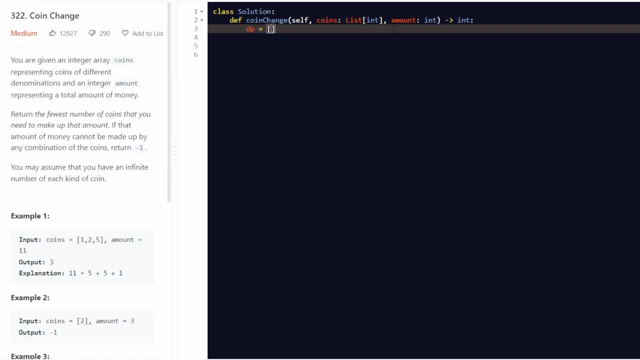 We'll use an array for this, where the indices of the array represent all the subproblems and the cell for each index represent the least number of coins needed to sum up to that particular subproblem. Index 0 will be initialized to 0, because that will be our base case. 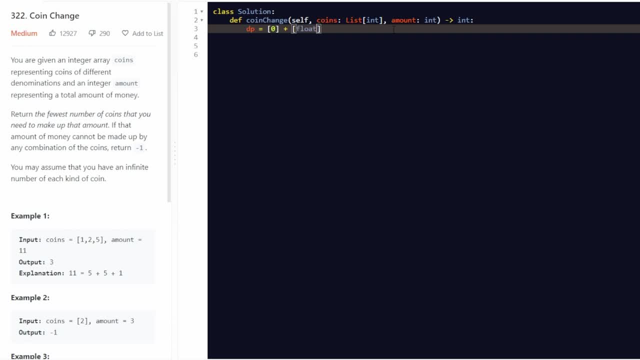 And the rest of the cells will be initialized to float infinity. That will just serve as a placeholder until we solve for the minimum of coins, And this will be the maximum amount of coins for a particular subproblem. Now we will start populating the DP array by first iterating through all the possible subproblems. 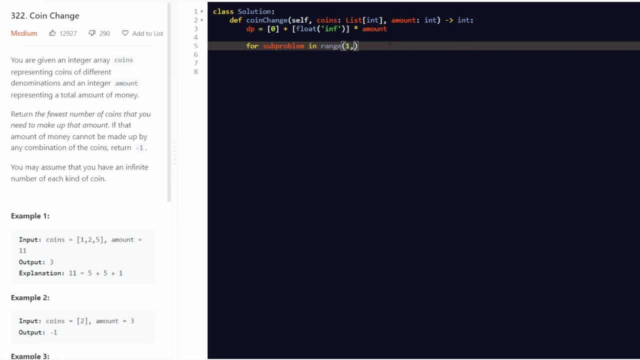 And that will just be all the values from 1 to. whatever the target amount is For each subproblem, we will try all the coins possible to see which coin will result in the subproblem And we will try to find the solution that has the least amount of coins. 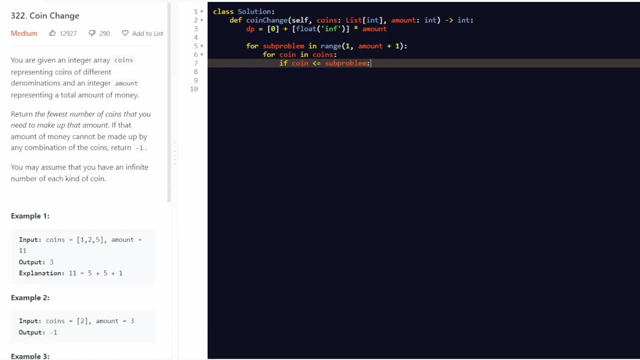 So if the coin is less than or equal to the subproblem we're trying to solve, then we can use it, And what we're going to do is we're going to see if that coin results in a solution. that is the minimum amount of coins for this particular subproblem. 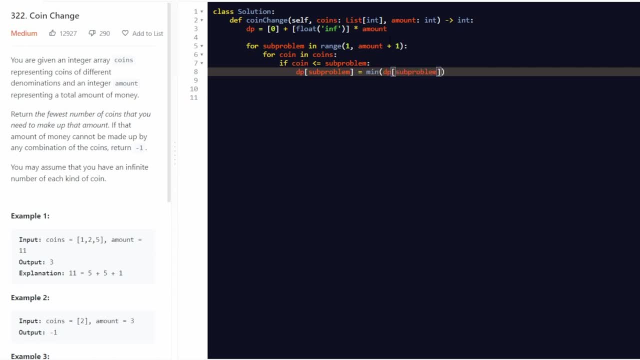 So what we're going to do is we're going to compare it against the current solution that is being stored in the DP array And then, if we want to use the coin, what we need to do is reference a previous subproblem that can be reached from this coin. 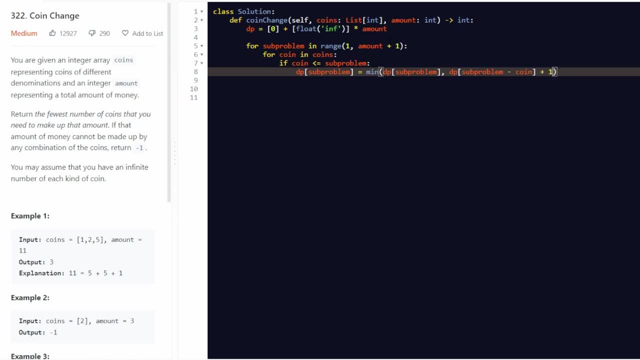 And since we are using the coin, we need to increment the previous solution for a previous subproblem by 1.. And then, once we do this and all the loops terminate, what we need to do is check the DP array for the target amount we can. 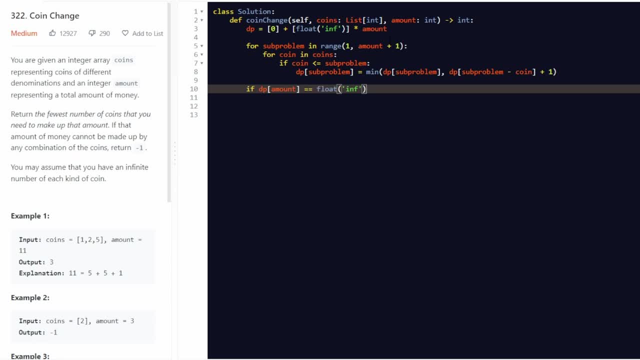 And if the target amount solution is set to float infinity, then we'll just return negative: 1. Because that means that the current combination of coins isn't able to solve to the target amount. Otherwise, we can just return the amount that's being stored at the end of the DP array. 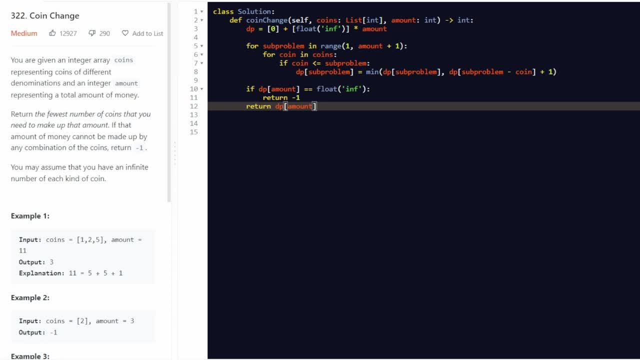 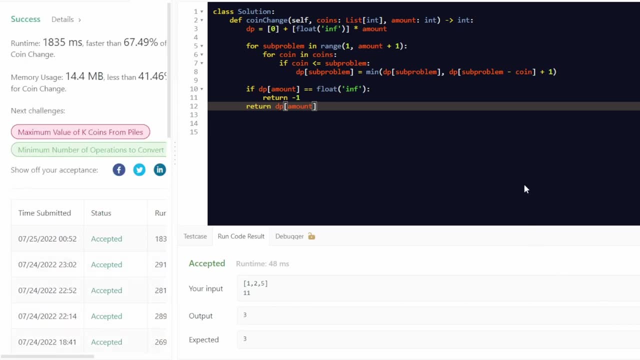 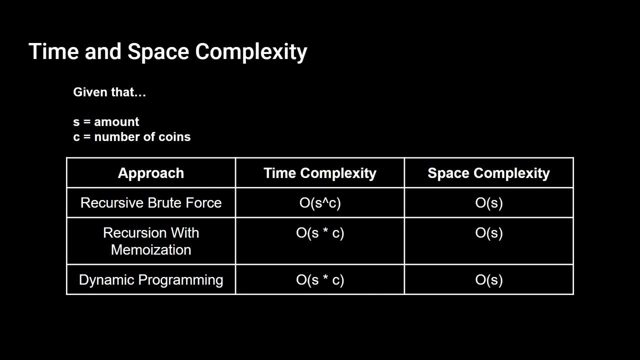 Now, what we're going to do is we're just going to run this And we're going to see it works, And this is the dynamic programming solution for coin change. Now, in order to talk about the time and space complexity of our different approaches, 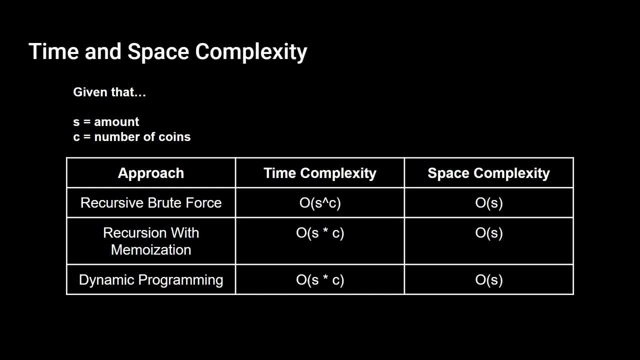 we need to consider both the target amount we're trying to reach and the number of coins we have access to. So if we let s equal the amount and c equal the number of coins, then if we look at the recursive brute force approach, the time complexity for it will be exponential.